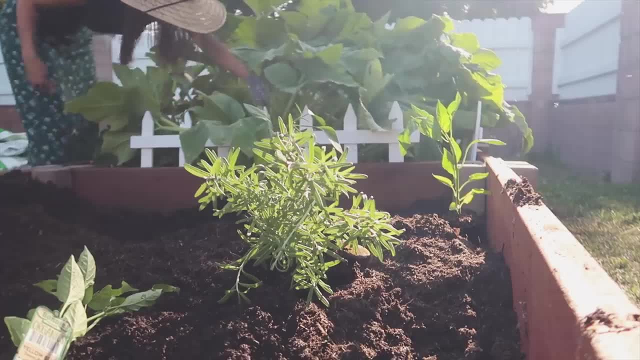 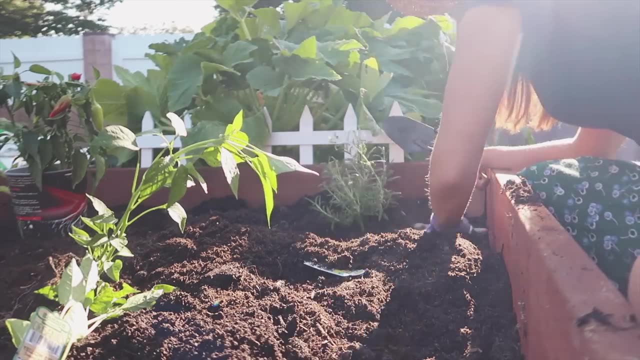 time to kind of share with you guys how I'm learning and what I'm doing to become a little bit more knowledgeable about growing food. Last spring we planted a full set of veggies and we just kind of went for it. We didn't start out with information, We just kind of picked the veggies. 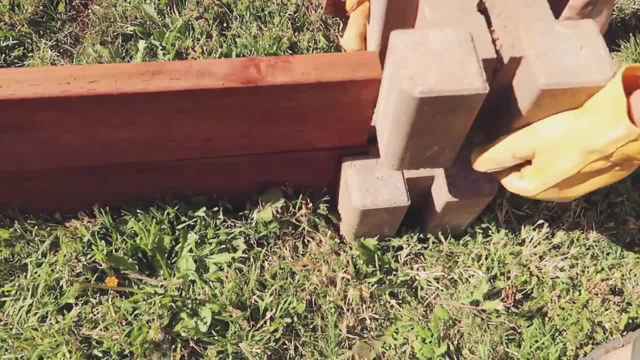 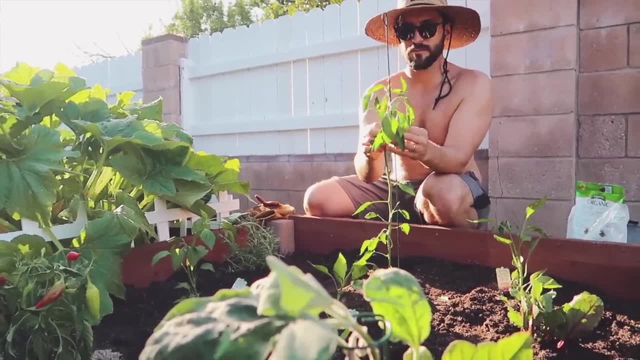 that we wanted to plant and we just threw them into the garden beds. We created these beds ourselves and I'll share with you guys exactly how we did that. We had some great success with this vegetable garden over the last year. I couldn't even believe. 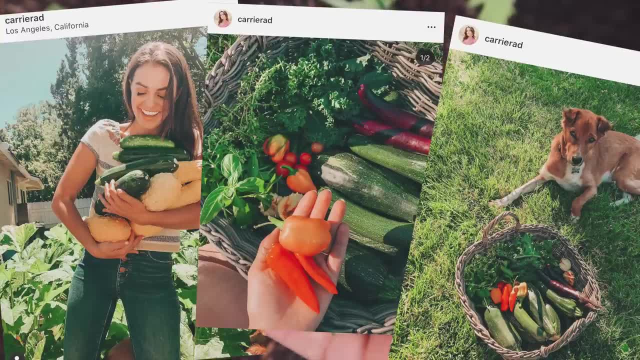 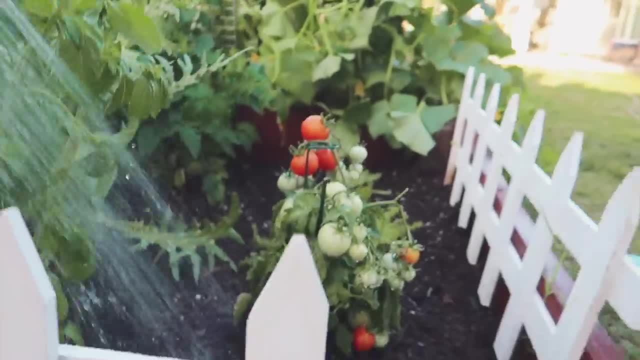 how abundant it was. but there were a couple of vegetables that didn't make it and that was primarily because we didn't do the prep that we needed to do to know what needed to grow next to what and when to plant what. The way that we look at it is that vegetables are like humans. They 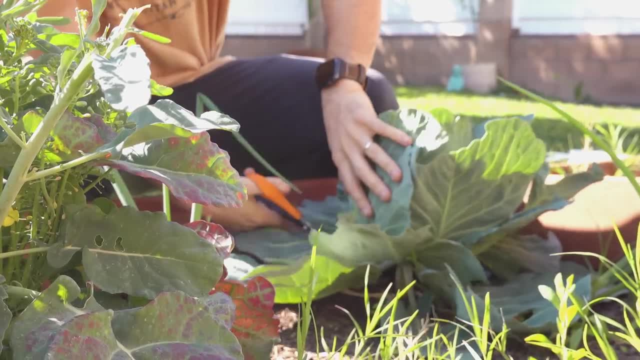 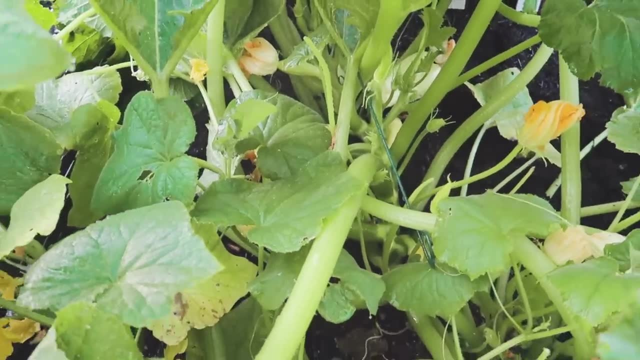 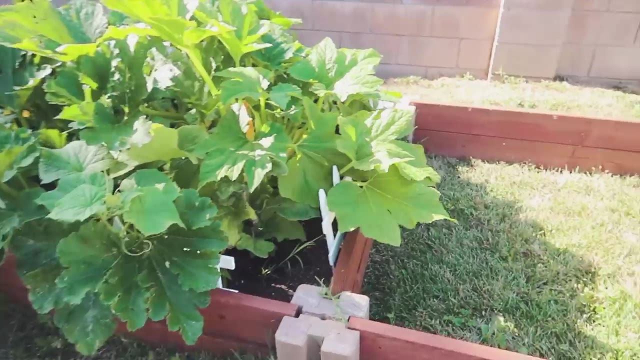 have feelings. They feel like other vegetables might be toxic to their self-growth, and so they want to be removed from them, And so you kind of just have to respect the vegetable's wishes and plant the vegetable where it feels the most comfortable. The most important thing we can talk about today is how we actually built the vegetable garden itself. 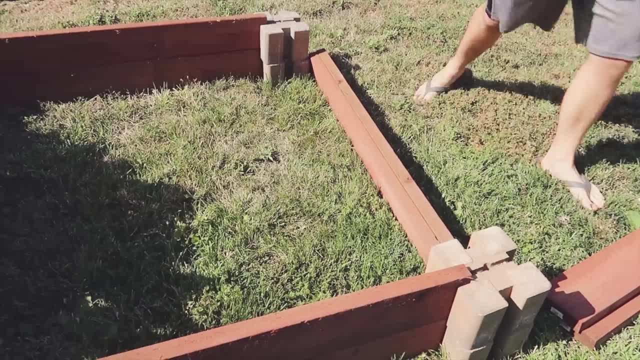 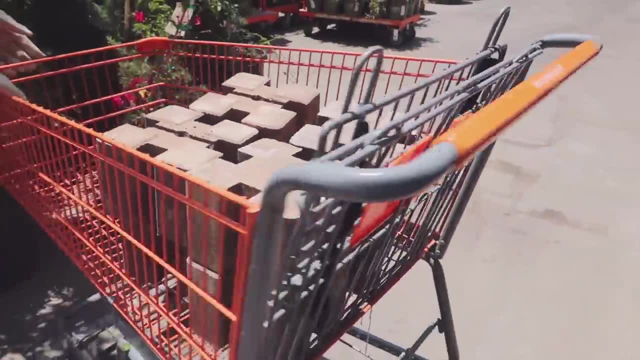 I got the idea from a sample that was in the garden section of Home Depot. I went in and I looked for each piece. It's pretty simple. You really only need three main things. First and foremost, this cement block with four cutouts on each side. 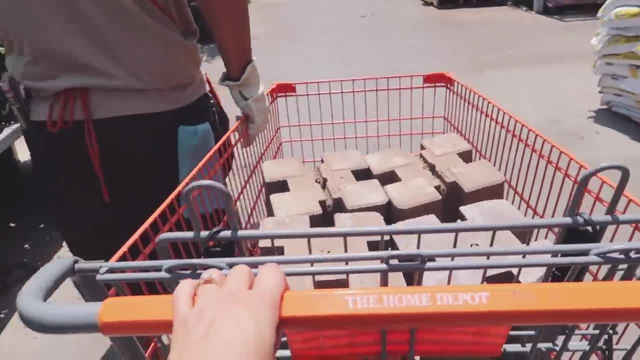 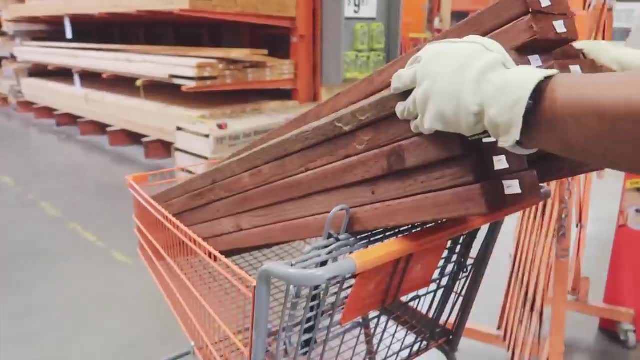 That you can find in the garden section. You can even screenshot this video or bring it in and show an associate and they'll take you the right direction in the store. Then I went inside of the store and I got these red wood planks and the gentleman helped me. 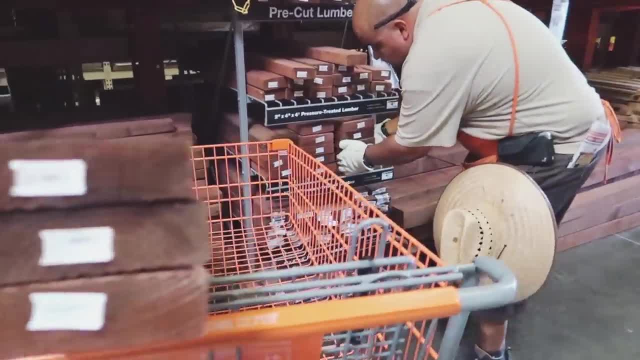 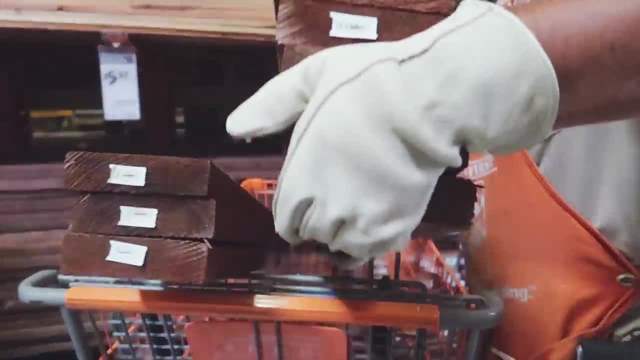 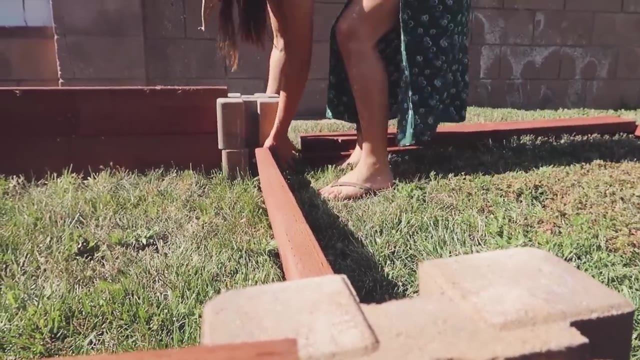 You'll want eight total and eight cement cubes total to make a raised garden bed above your grass. Now, when we ended up expanding, we actually ended up taking the second store. We actually ended up taking the second store Off and adding it to expand the garden itself this time around. 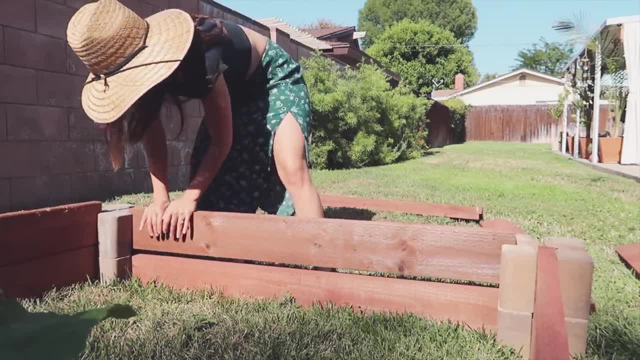 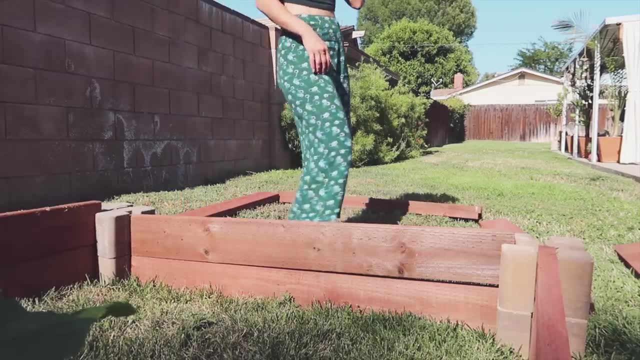 But I want to show you guys all the different options because there are different ways that you can do this. So you'll want eight cement cubes and eight red wood planks to create one plot. Now, if you want to make a bigger bed, then you'll want to double that up as you go. 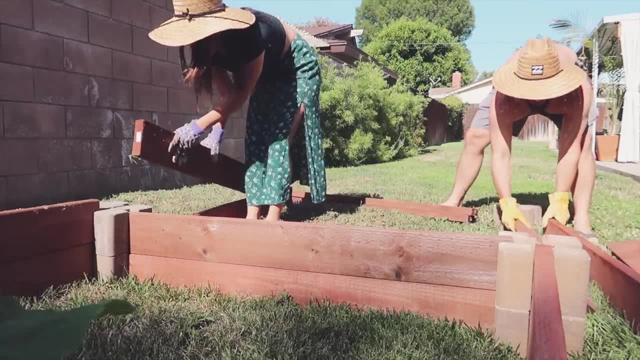 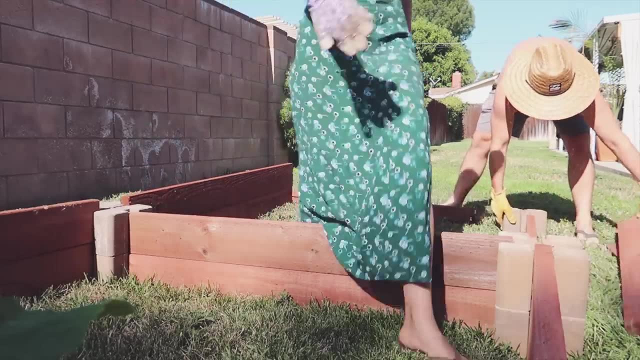 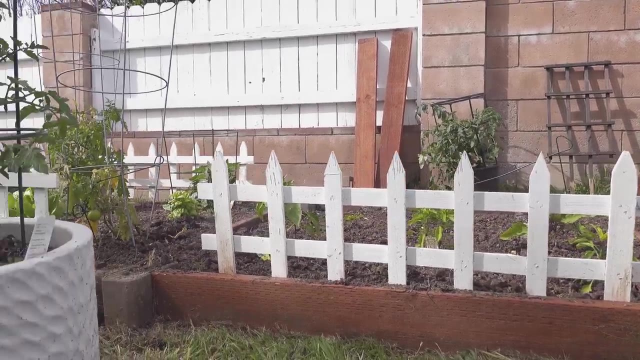 Something that we did do recently, this time around, was that we wanted to expand, but we didn't want to go get more cement and more wood. So we actually took the second story off and we expanded it that way so that it just wasn't as tall, and it's really been working for us perfectly. 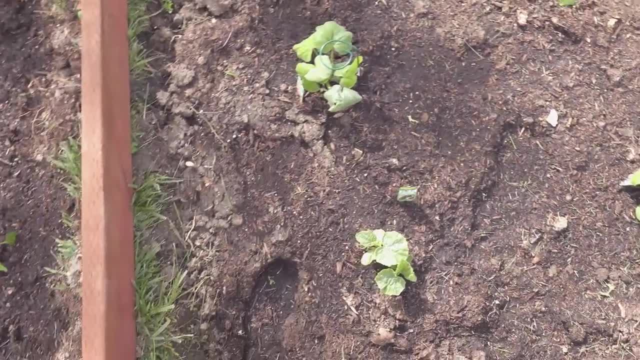 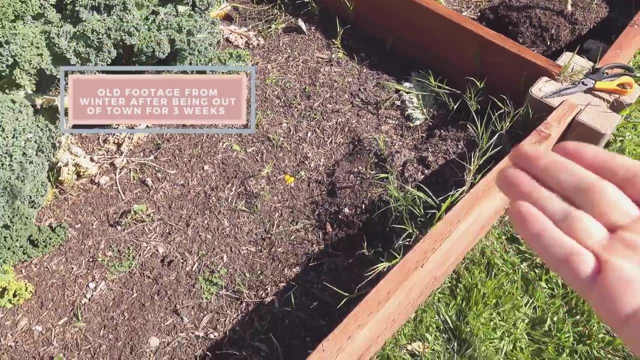 It's just based off of preference and kind of how you want it to look. As you guys can see, we have grass growing through our soil and some people put plastic underneath their soil or some sort of material to stop the grass from growing through. 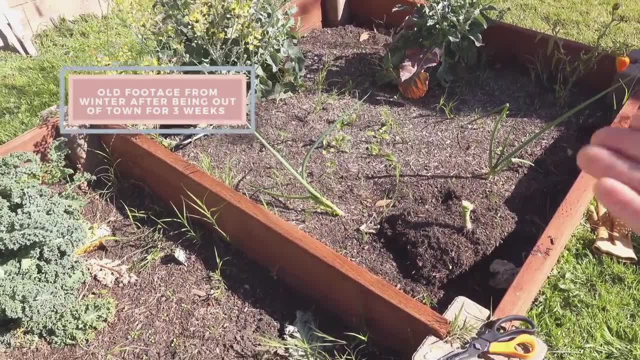 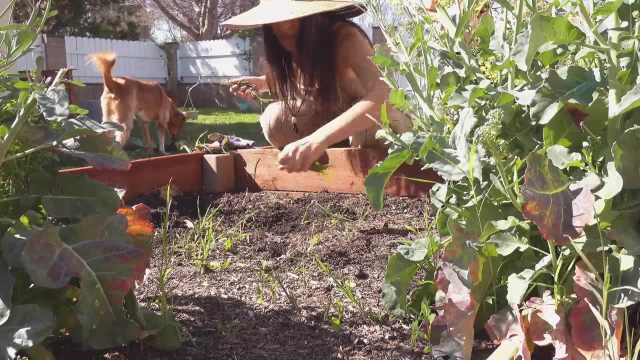 We tried that on that one And it became. It became kind of swampy over there and we didn't like it. We prefer just pulling the grass when we see it. Obviously this is a little bit more work, but we enjoy it. 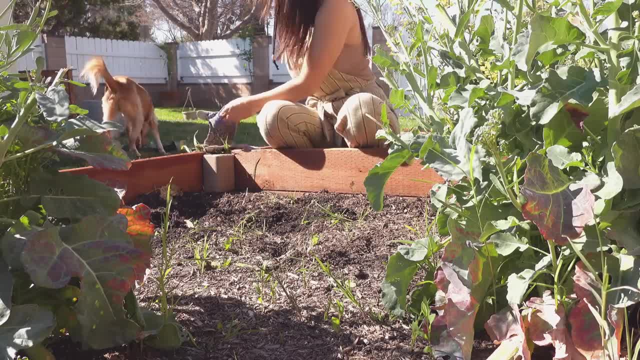 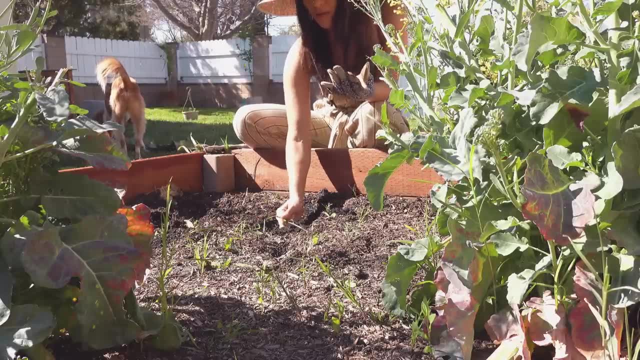 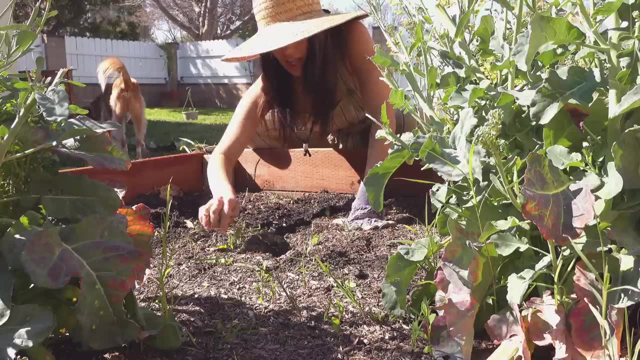 So we just pull it when need be. Sometimes it grows a little bit faster than we can get in there and do because we haven't been out here in a while. But right now, you know, I'm going to go in there and pull all these and I'd say I pull the grass maybe about every three weeks. 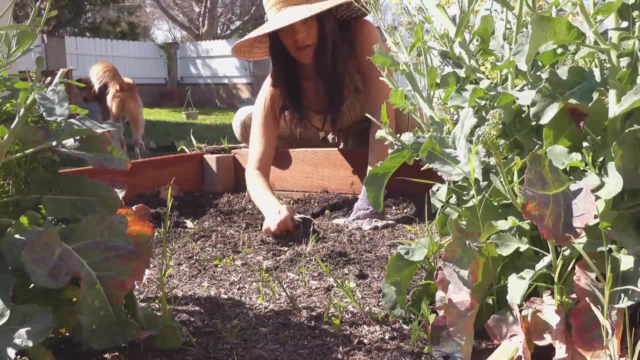 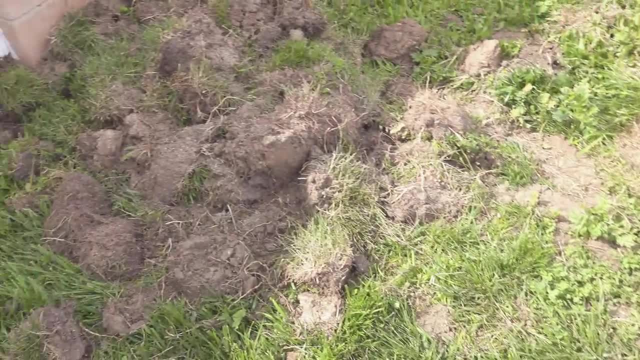 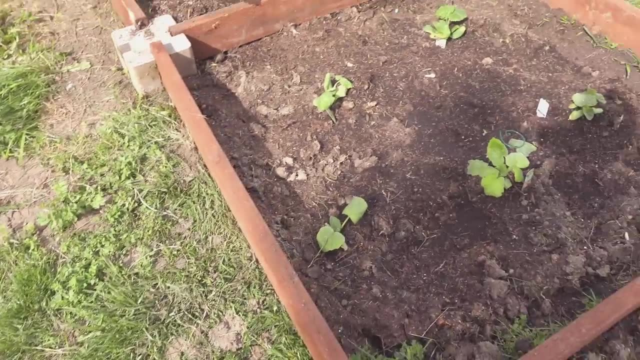 I don't know if it grows through and we just like it this way. So it's it's preference and in how you want to do it. Another option is to remove the grass completely from the inside of the garden bed. So Alex took a shovel and he removed all of that grass and threw it outside of the square. 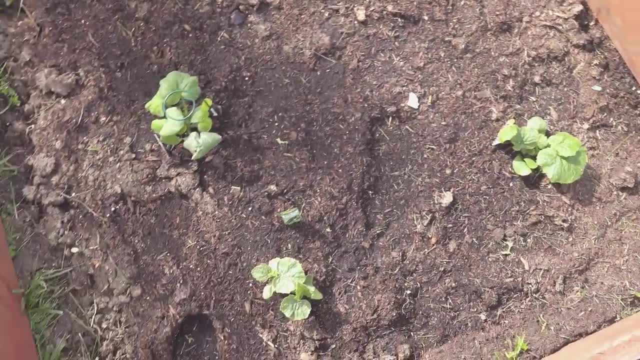 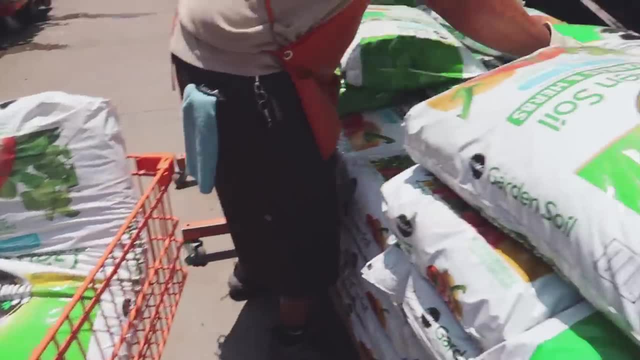 And then we put the garden soil over it and added the compost soil as well. This is a little bit less maintenance. So, if this is interesting to you, Alex has a video going up on his channel in about a week Where he explains exactly how to do that. 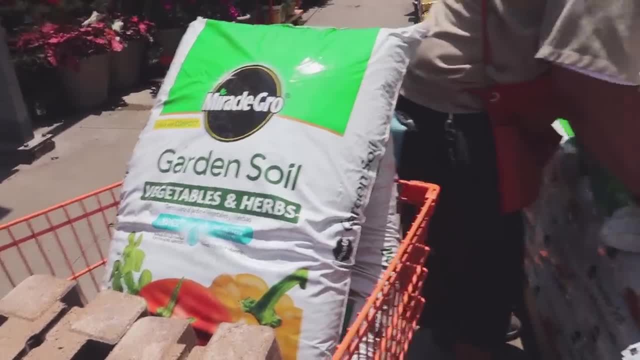 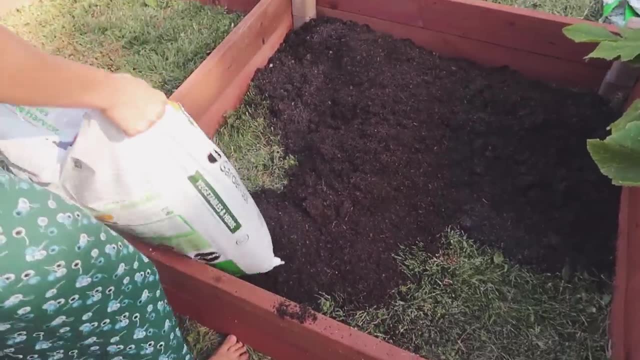 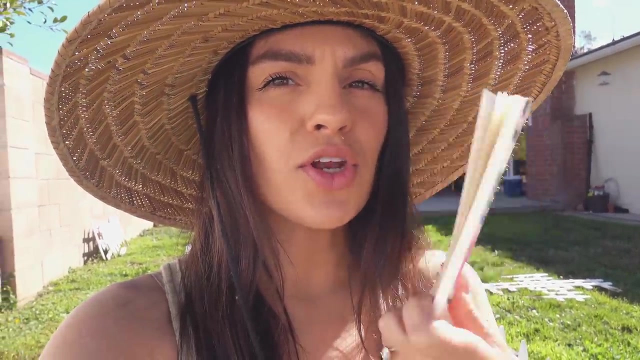 So stay tuned for that video. And the third important item that you can get from your local garden store is your garden soil. We use a Miracle-Gro garden soil and we use about four packs of garden soil per square. The next thing I would recommend is to have some type of garden notebook. 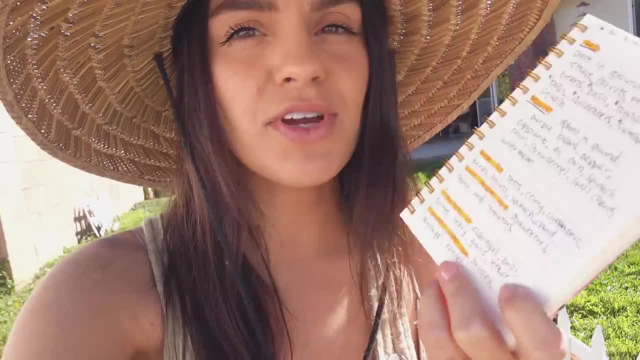 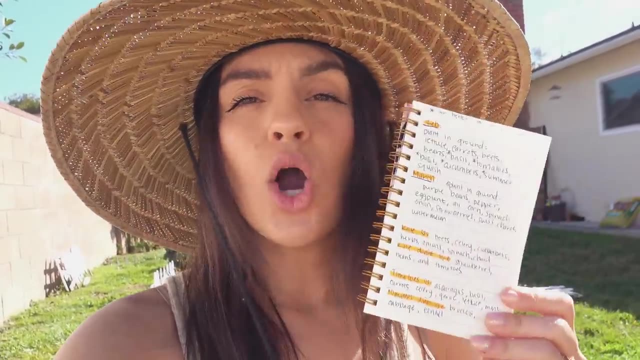 I like a small one that I can throw into my purse, that I can bring to the nursery And I have some garden notes here. You can do some research, Look online or in books To figure out exactly what the best vegetables are to plant at what time. 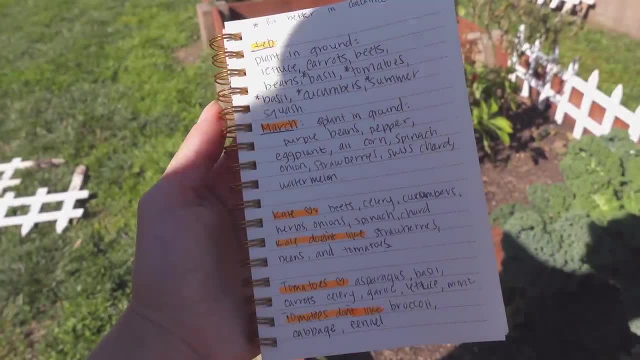 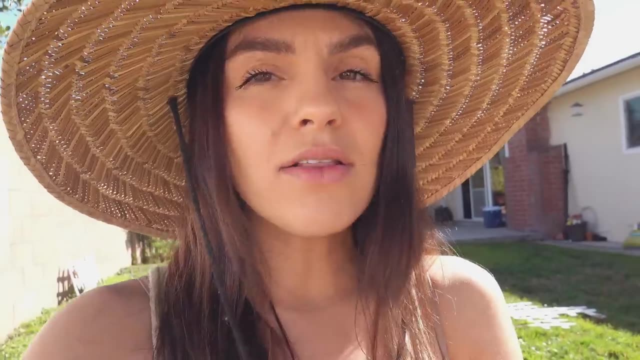 So I've gone ahead and done that for February and March this year, depending on what we plan on growing, And then I also put some notes down at the bottom here, talking about what kale loves to be next to and what it doesn't like. 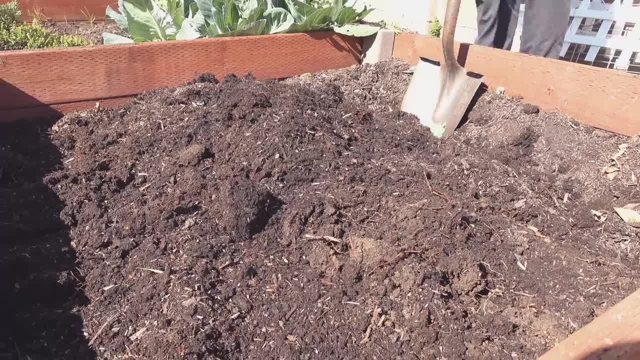 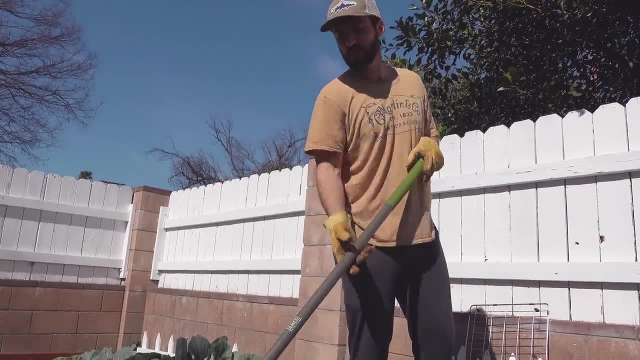 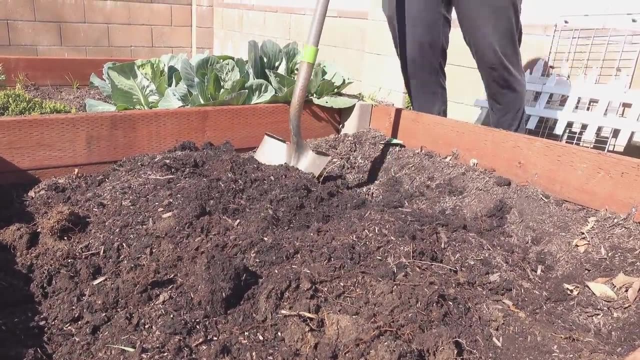 What tomatoes like being next to and what they don't like. We've kind of left this plot fallow for most of the winter, And so what we need to do is: This was a very productive patch of zucchini and summer squash, So what we're trying to do is stir the soil up. 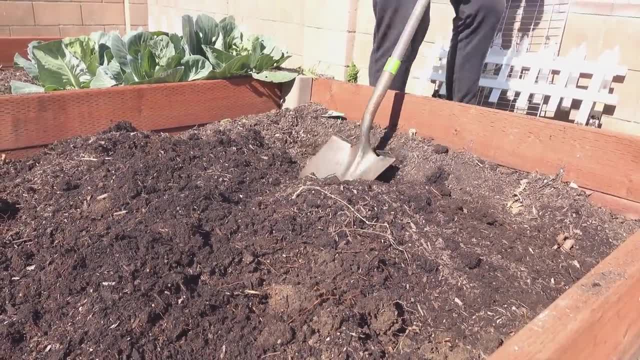 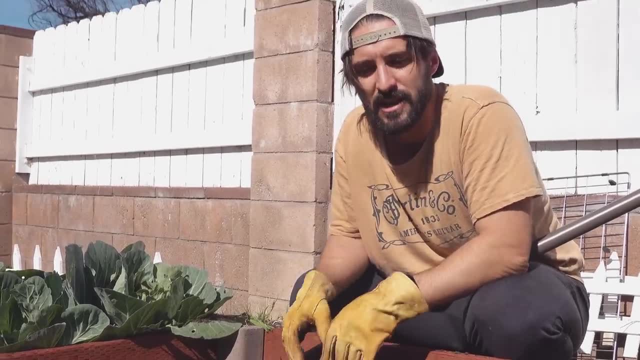 Get everything moved around, Make sure that these root structures from grasses and stuff are as cleared out as possible. Now we're just trying to till the soil and mix it all up, Because it's not good for soil to just like sit static for a while. 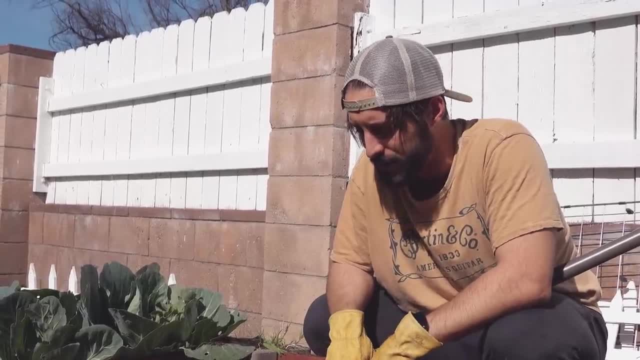 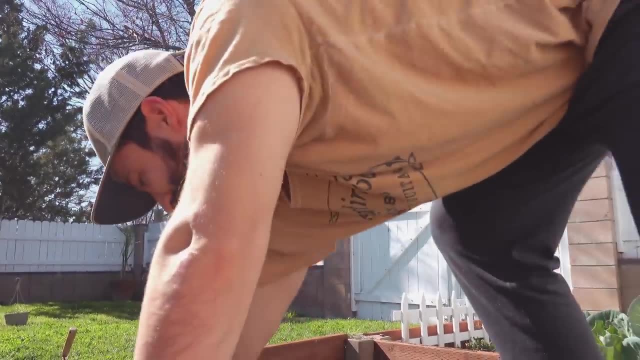 You get pests and stuff Trying to grow in there. We've pulled about six or seven caterpillars out so far, But a good sign, the soil is super healthy, There's a lot of earthworms And we're just going to mix it all up. 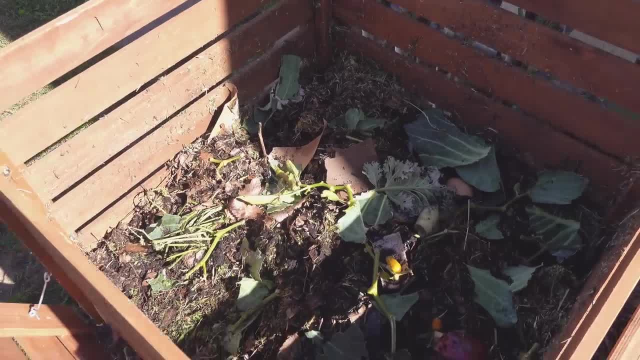 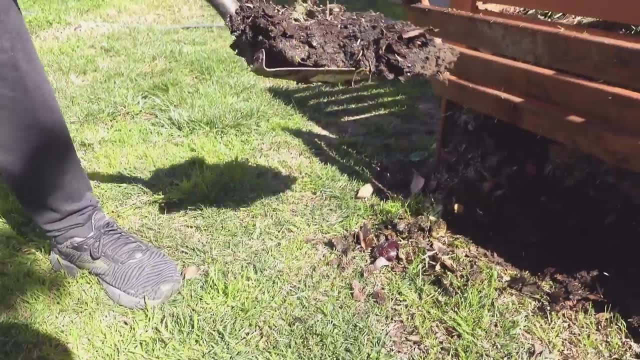 And then we're going to add some of our compost, which we've been making for the last six months, And we'll mix that in here and in a couple of days we'll plant some stuff. It's like a natural fertilizer. It's a natural fertilizer and natural pesticide. 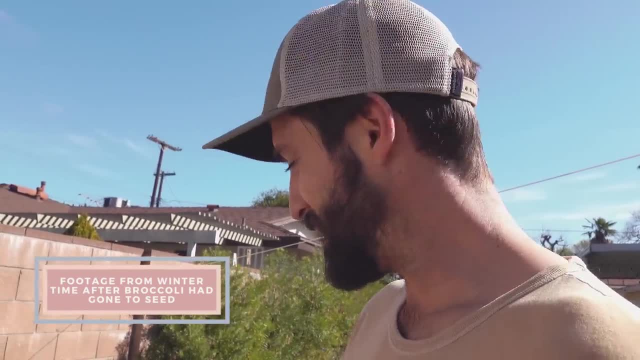 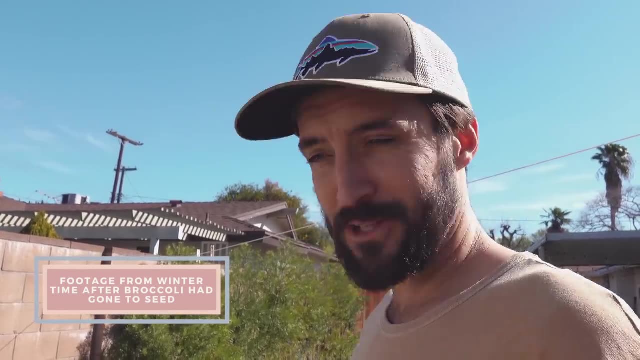 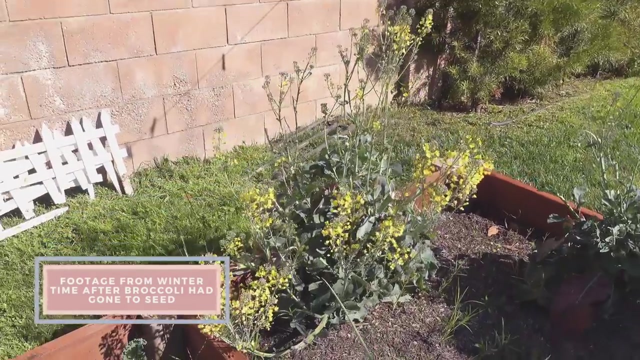 I think it's time to say goodbye to that, Say goodbye to the broccolini. It's been good. We harvested quite a lot of broccolini. I don't even know any, It's very broccolini-ish, It's flowering. 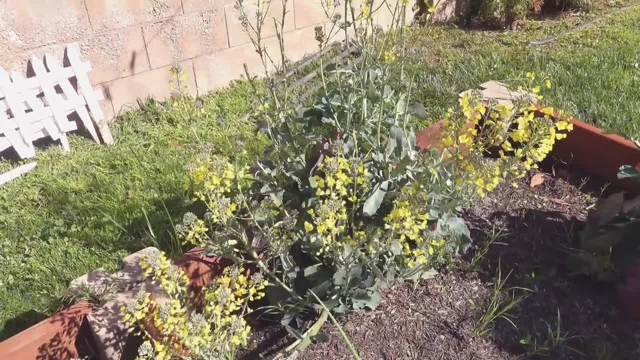 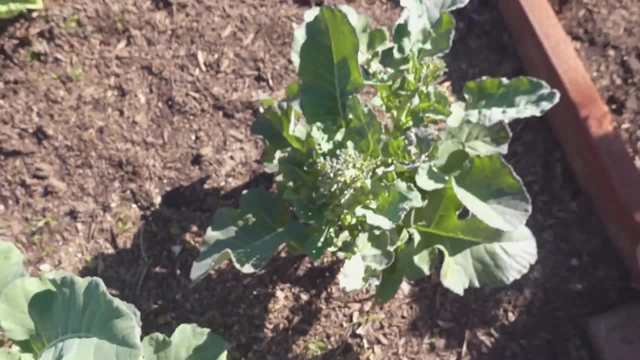 It's just gone to seed. I tried to trim it down about a week ago, but it's still just putting everything to seed. This is current time footage of our garden, And when we removed the broccoli that had gone to seed, We replanted. 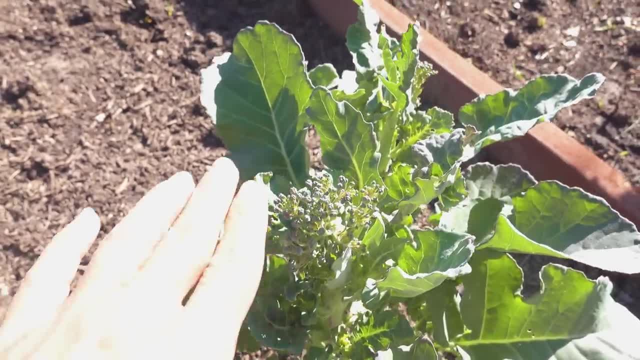 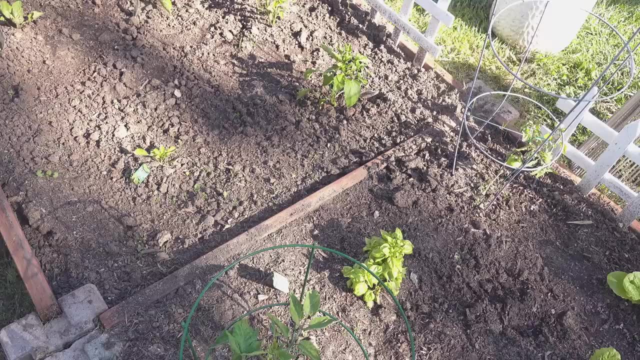 So, as you can see, we already have more broccoli growing. In a couple of weeks we'll be able to eat this. I love growing broccoli. It's so hardy and it grows so nicely. I'm going to show you guys some more vegetables that we planted and that we have going this time around. 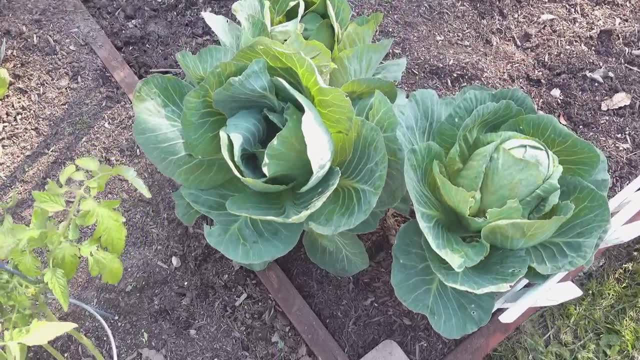 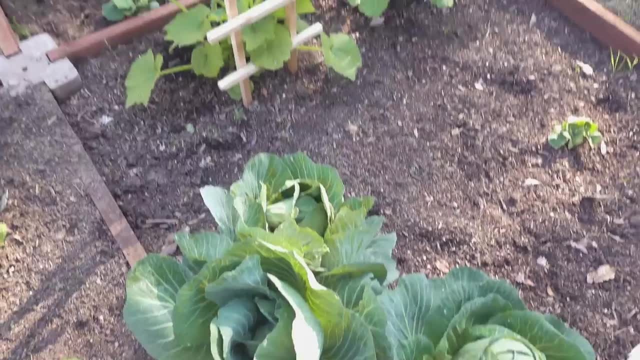 The cabbage we planted in the fall And it has been so abundant. We have gotten so much cabbage from there And we have more growing in This. one should be done soon. We have zucchini growing there. We loved growing zucchini last spring. 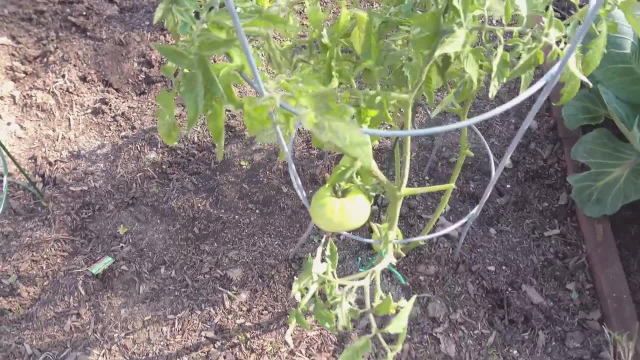 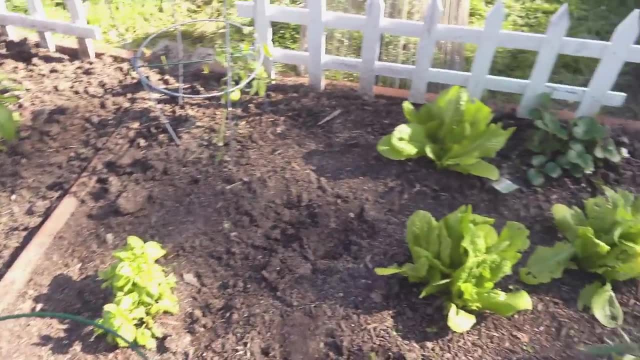 So I can't wait until that starts coming in again. We have tons of tomato plants going. I love having tomatoes because we eat so much of it. There's another tomato plant there. We've got basil, Some lettuce and some strawberry over there. 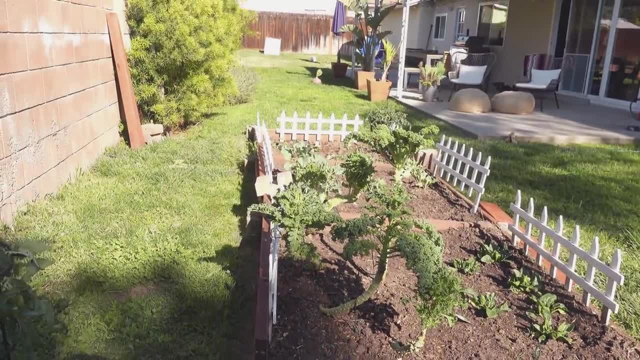 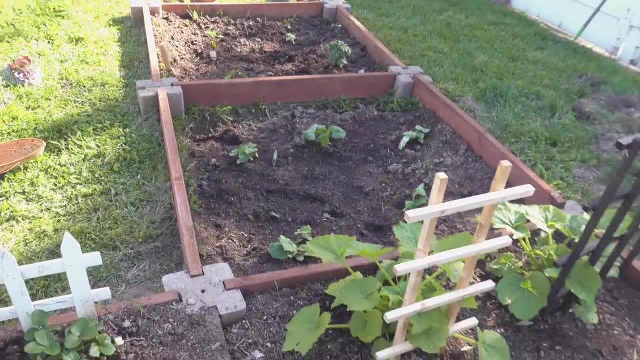 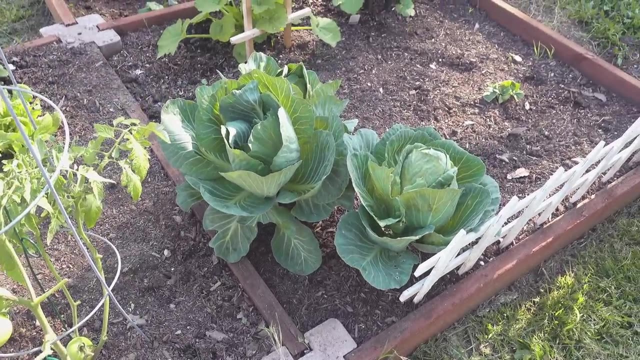 We've got peppers and kale and spinach and cauliflower And the broccoli I already showed you guys, And then over here we have cucumber and zucchini that will be growing. We just need to give it some time for this new season. But as we wait, we have some others coming in, like the cabbage and the broccoli and the kale and the spinach. 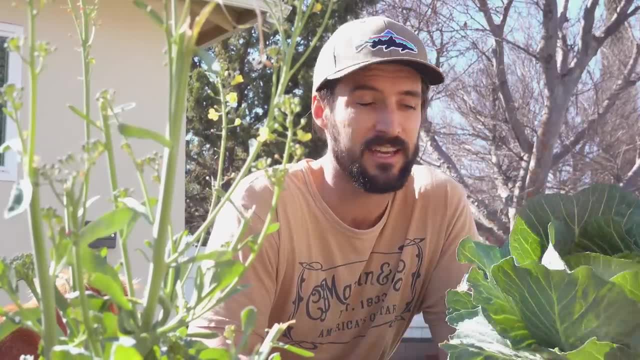 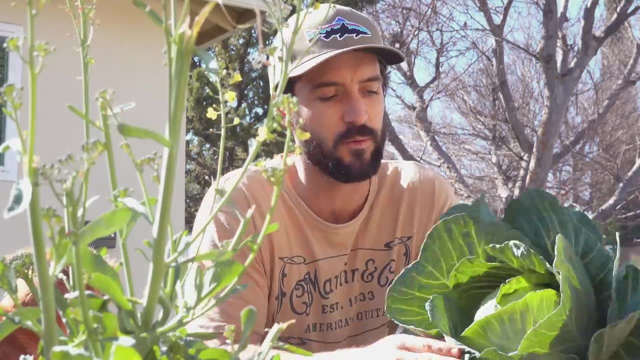 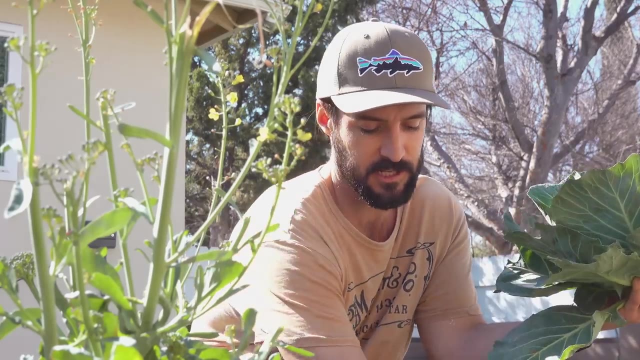 So this is kind of the fun part. We are harvesting the winter crops And the cabbage actually did really well. We've never grown cabbage before, But we have a whole cabbage patch over there that also needs some attention, But it's cool. 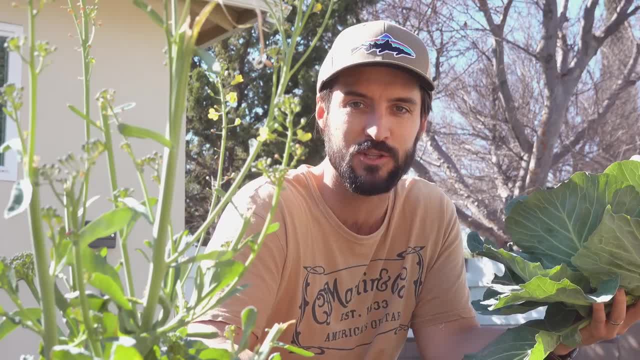 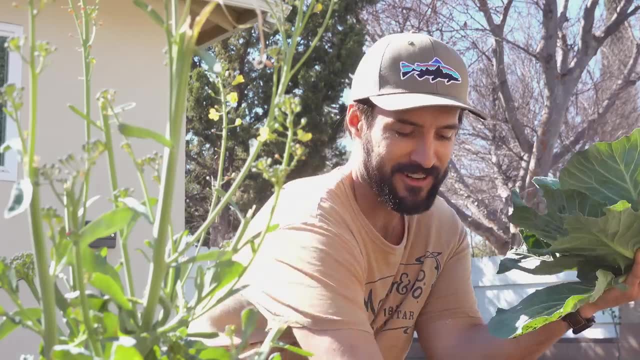 It's like you're harvesting one cycle and then you're comparing the soil for the next one And there's something really like. It's a strong metaphor for life. you know You've got to harvest what you can and then grow some more. 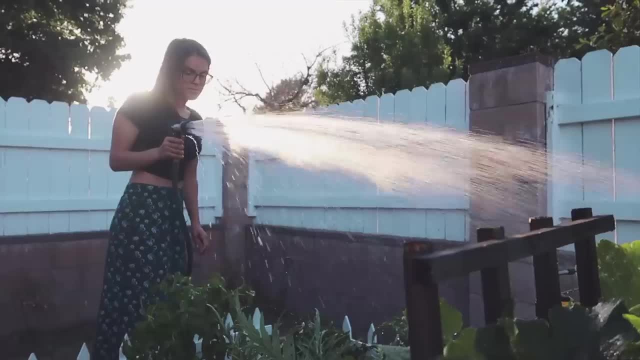 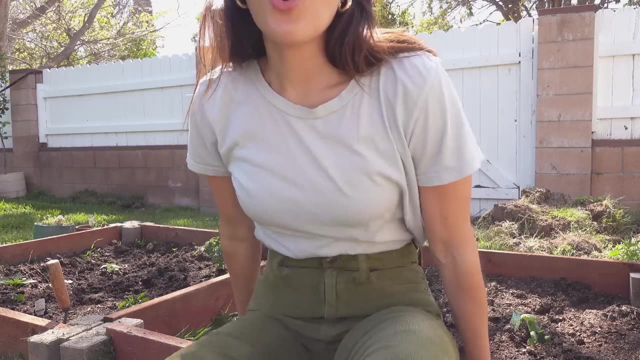 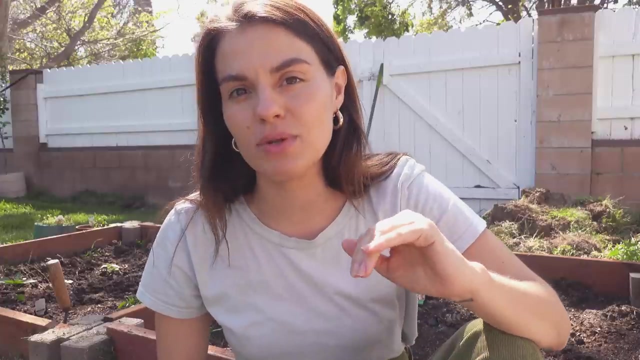 All right guys, so I hope that this video was helpful to you in some way. At least, it gave you the basic information that you need to have a backyard vegetable garden. Now, of course, there are tons of different ways that you can go about it. 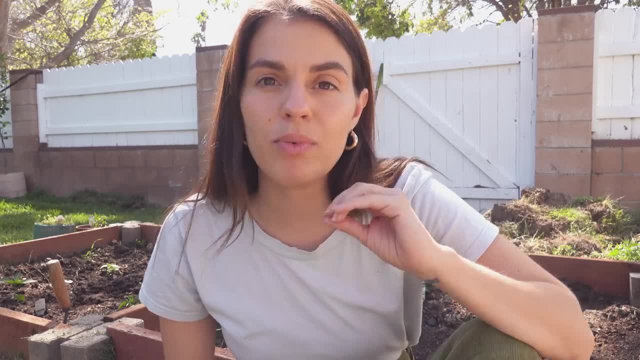 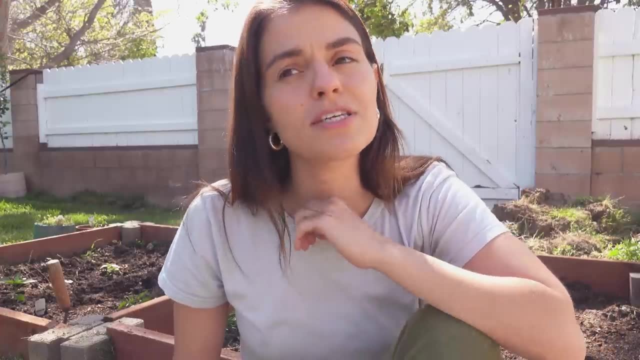 We have a grass lawn, so we've learned how to do it with what we have And, as you guys can see from the video, we tried different things out and we've learned so much along the way. I mean, you learn something every single day when you are growing food.